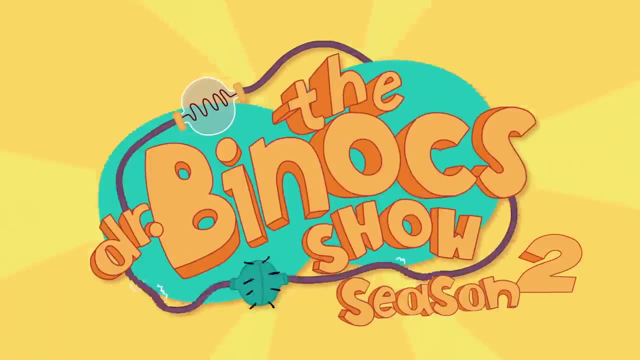 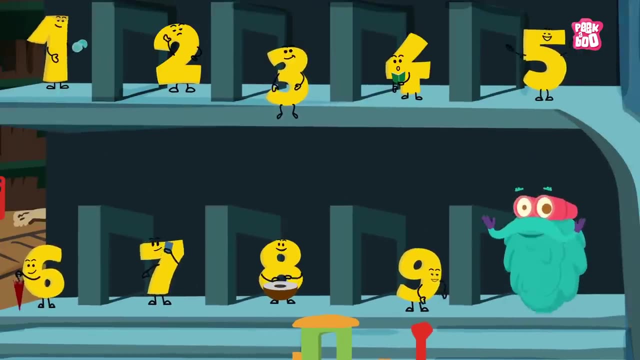 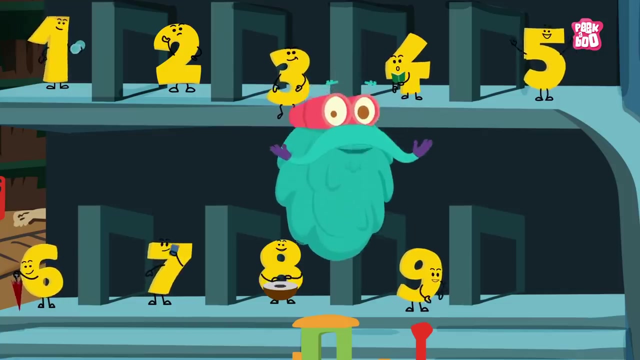 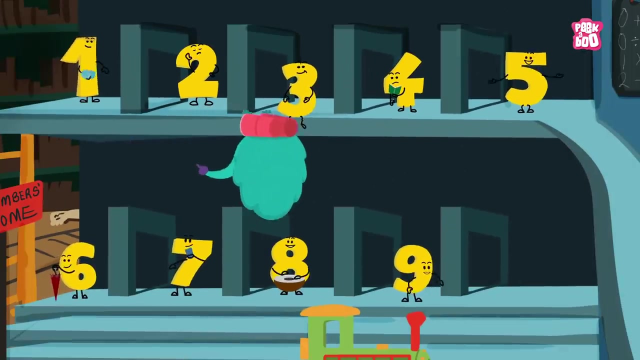 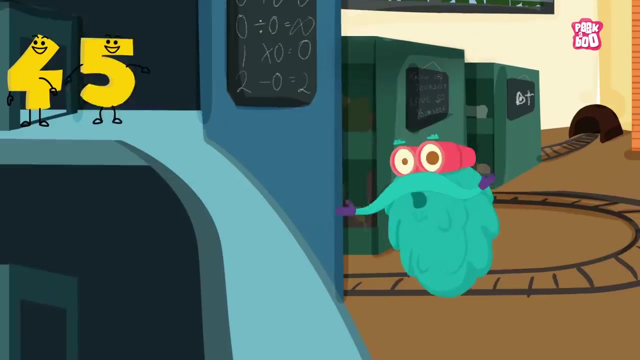 And it's complete. Oh, you're back, I've missed you. So what do you think of my new collection of numbers? Huh, Something is missing. That's impossible. Everything's here. There's nothing missing. Oh wait, Now I see. 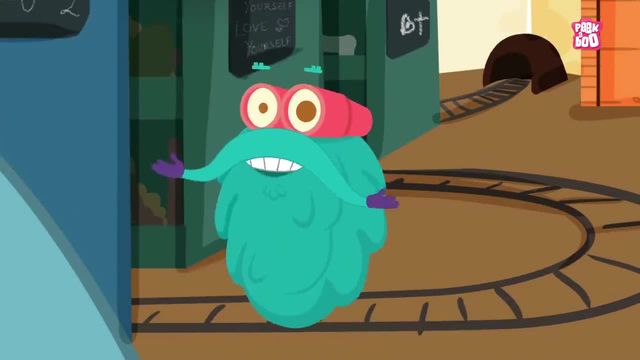 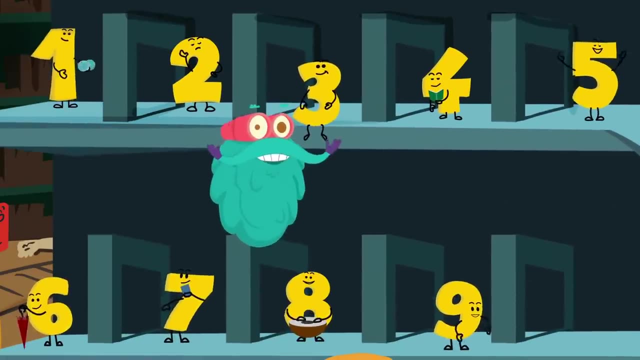 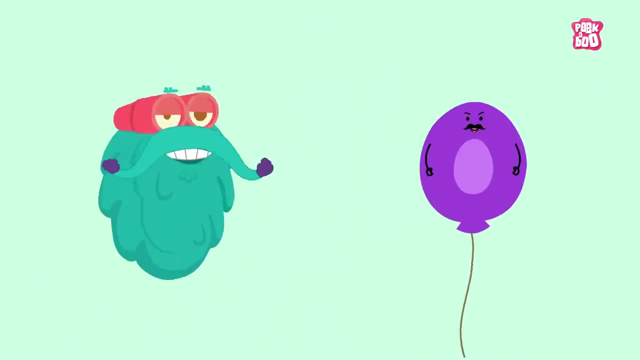 You are talking about the number that denotes nothing. You are talking about the number zero, right? So let's zero in. Oh sorry, I mean zoom in. Don't you wonder Why the number zero is so important in mathematics, when it only means nothing? 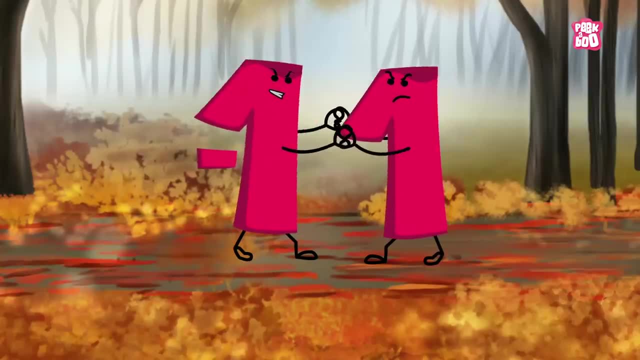 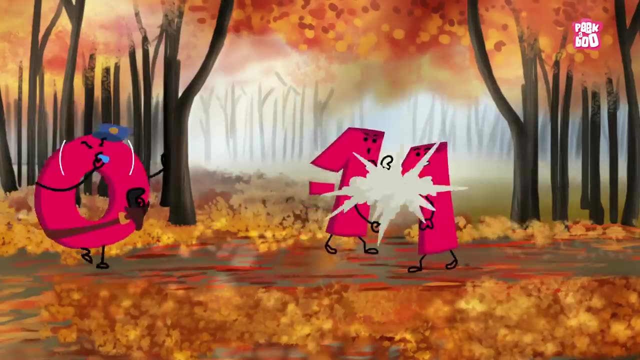 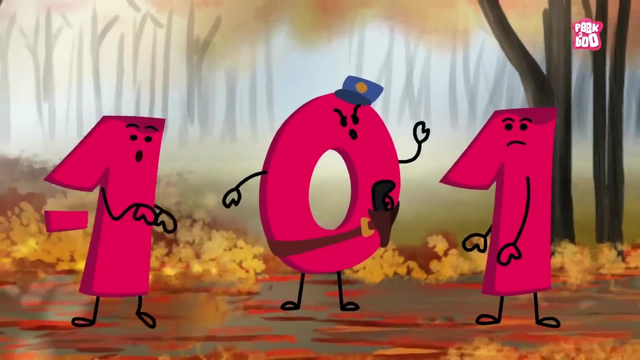 Well, kids, it's because of the two very different and very important purposes that zero serves. Firstly, it's zero that separates the negative numbers from the positives. Secondly, it serves as a placeholder for writing numbers. Consider the number ten, for example. 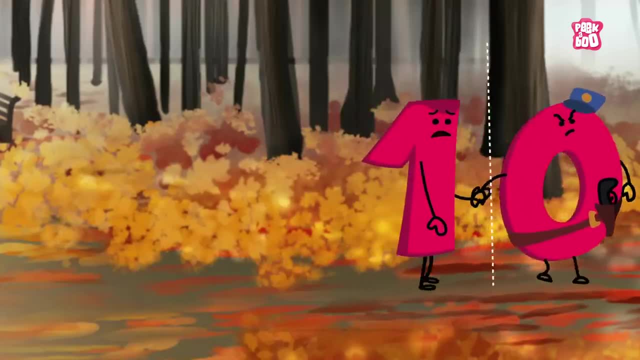 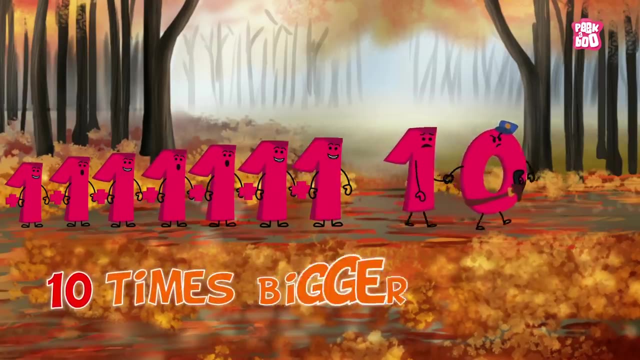 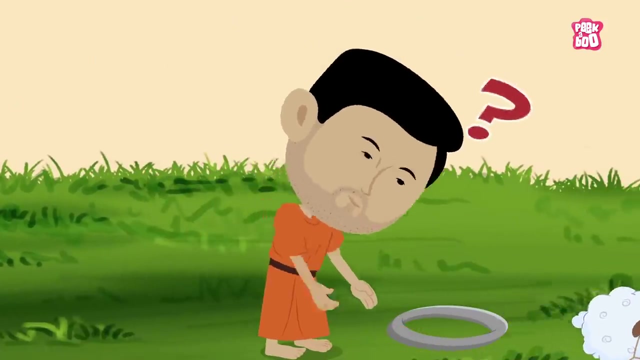 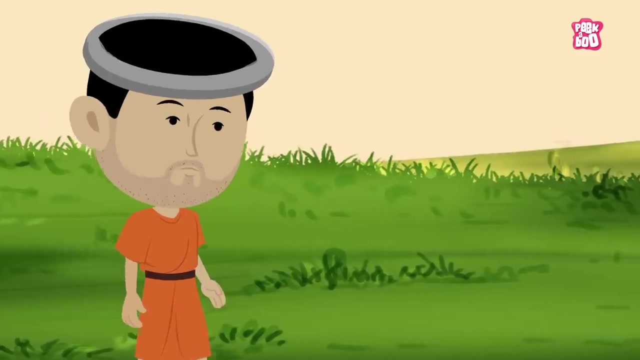 It has two parts, one and zero. The number zero is placed here to say that it is ten times bigger than the number one. However, people from ancient times could not wrap their heads around the idea of denoting nothing by something, So they never considered zero as a number. 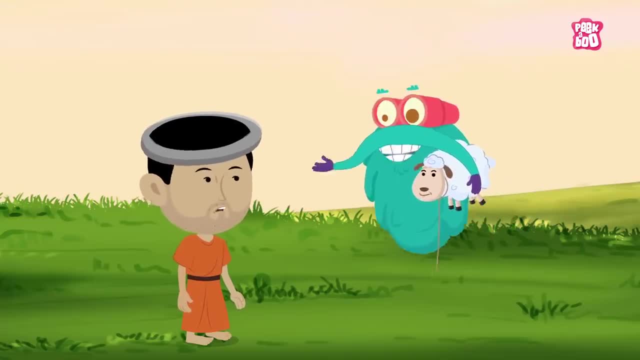 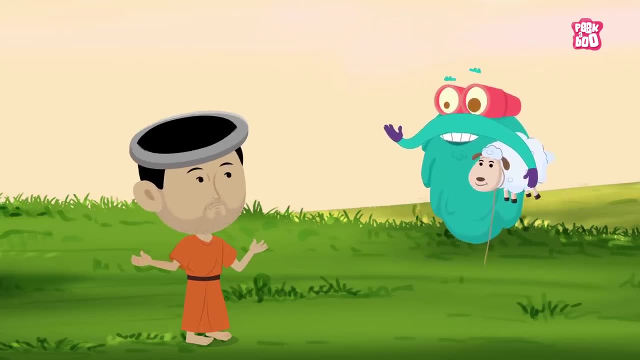 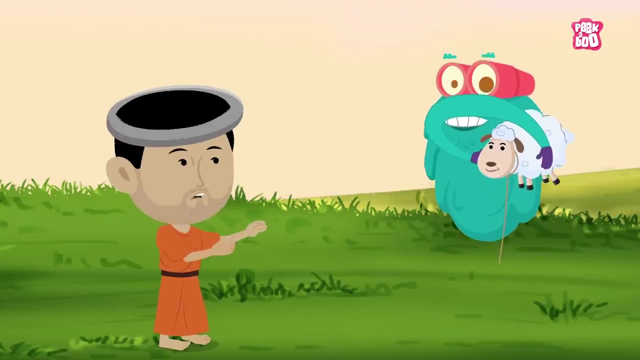 Consider this man, for example. Excuse me, sir, Will you please tell me how many sheep you have now? I don't have even one sheep. You see, people were able to communicate the idea of nothingness One minute, sir. 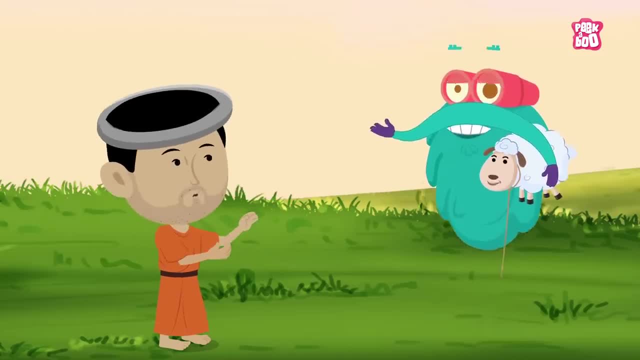 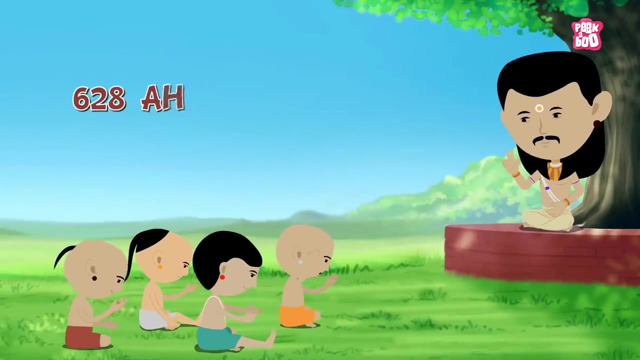 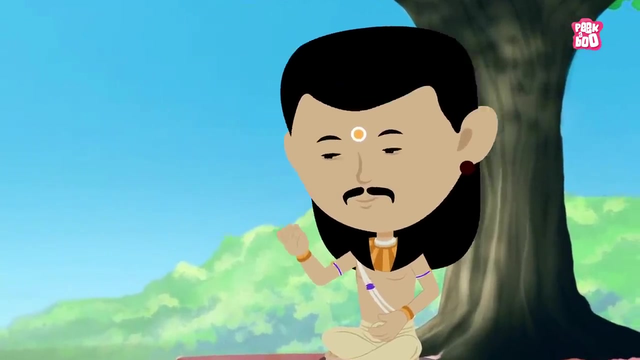 But they did not have a representation for it. What is it, My sheep? Oh yes, of course I'm sorry. Here you go. It was not until 628 AD that zero became an important part of the number system in East India. 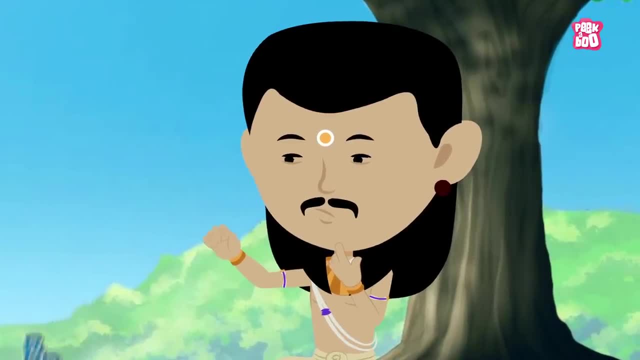 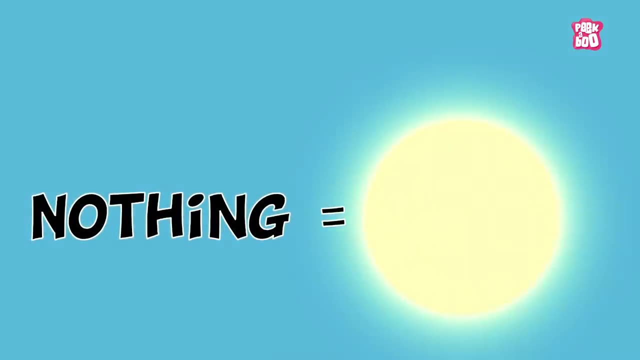 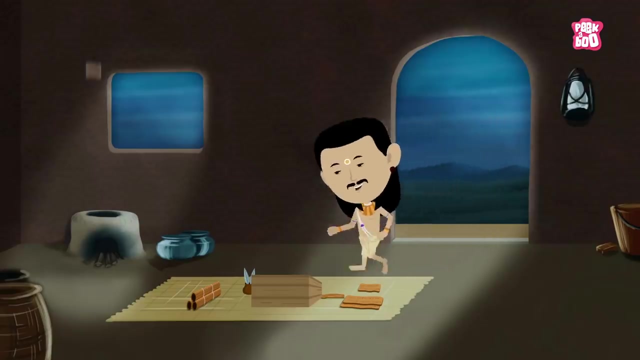 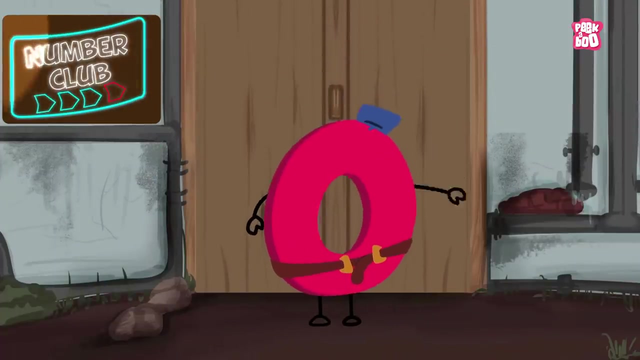 An Indian astronomer and mathematician, Brahma Gupta, took the idea of nothingness, symbolized it with a dot and included it in the number system. This was the first time in the whole world that zero was included in the number club. 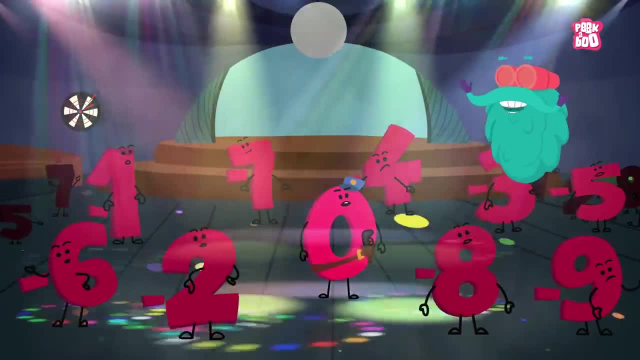 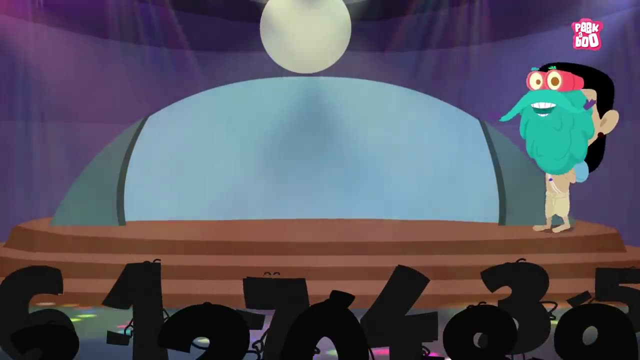 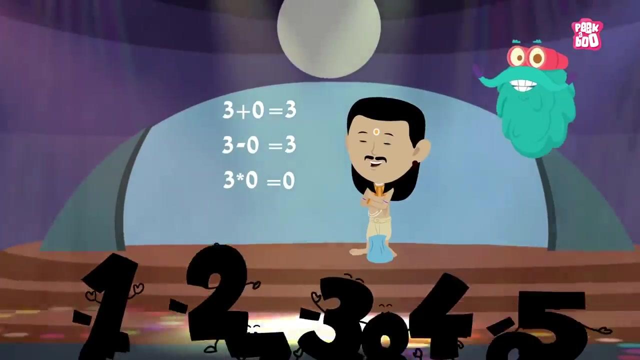 Hey, hold on, Hold on. Hey, wait a minute. Not so fast with your celebrations there, peeps. Although Brahma Gupta gave us the rules for using zero in calculations, defining its very first important use, he never introduced zero for its second purpose. 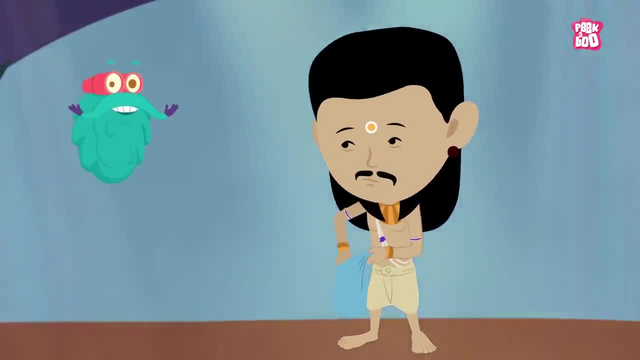 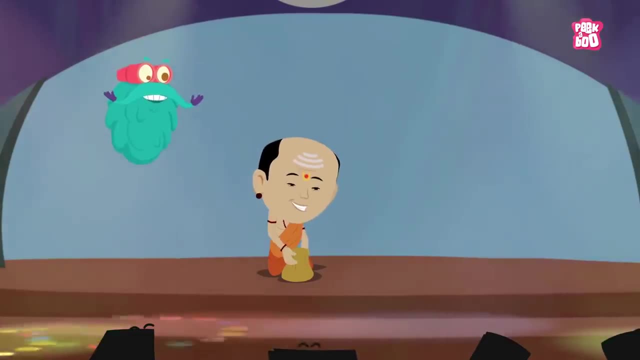 That is, as a placeholder digit. It was another Indian mathematician, Aryabhatta, who gave rules to use zero as a placeholder. This helped representing numbers like ten with one and zero, instead of coming up with a whole new symbol for them. 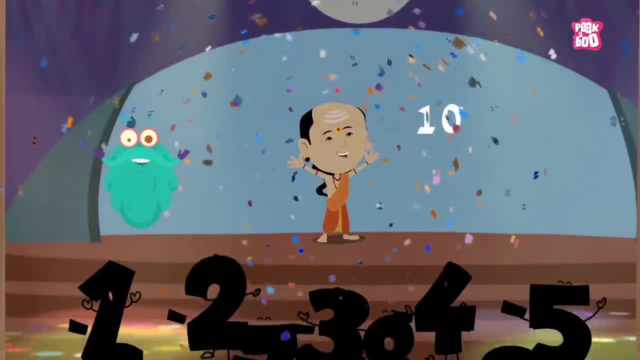 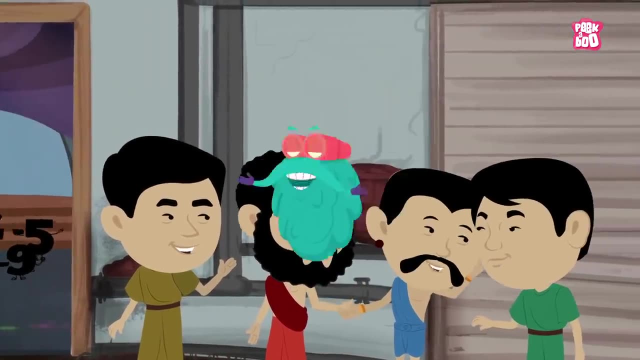 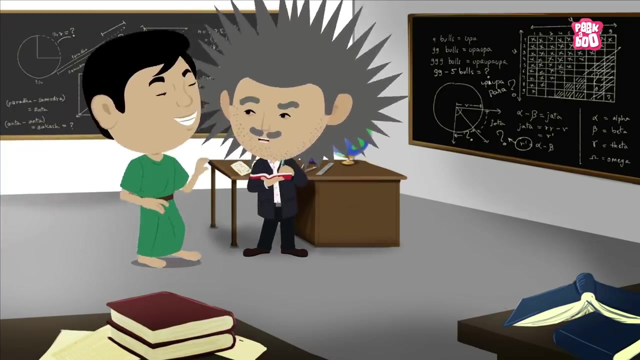 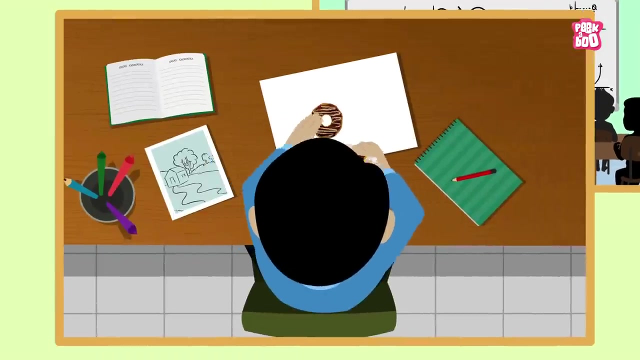 Thanks to these mathematicians- for nothing I mean zero- Soon this revolutionary knowledge spread around the whole world, and mathematicians across the globe started using it in their calculations. Today, zero also forms an integral part of physics, chemistry, astronomy and computer science too. 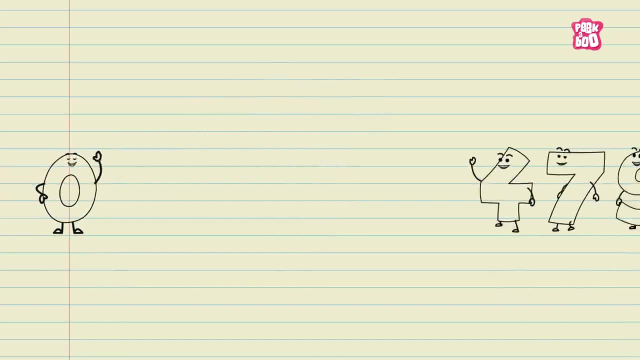 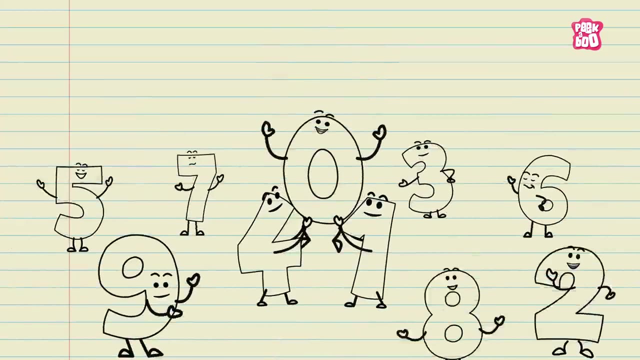 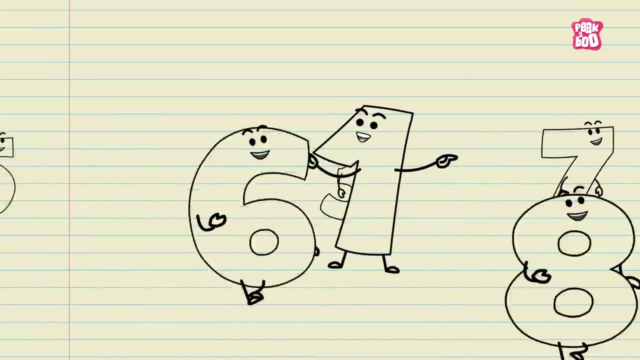 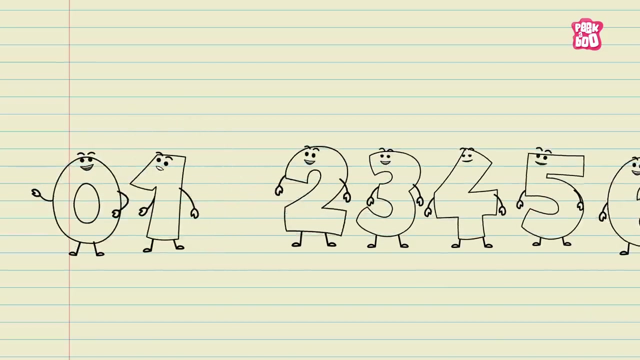 Whoa, Welcome, welcome. We have been waiting for you all: A family of numbers with the hero zero. So now let's look at some of his properties. When the integers are placed on a number line, number zero places itself before number one. 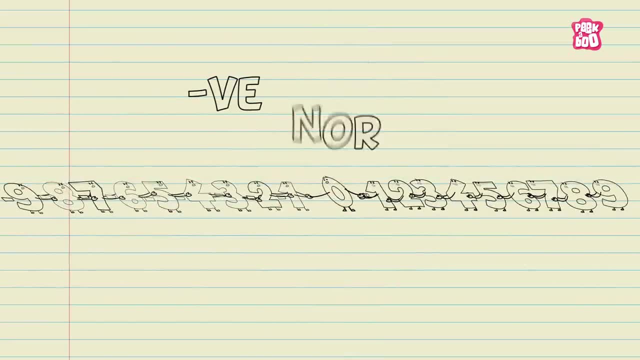 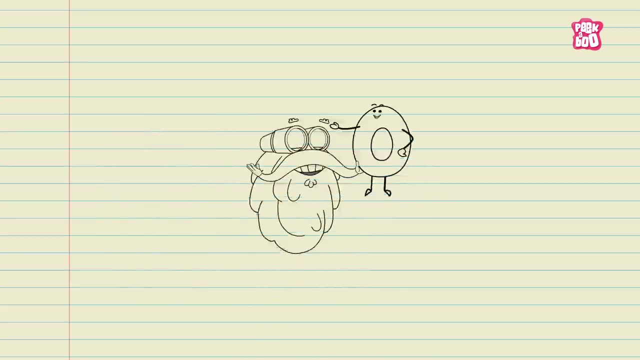 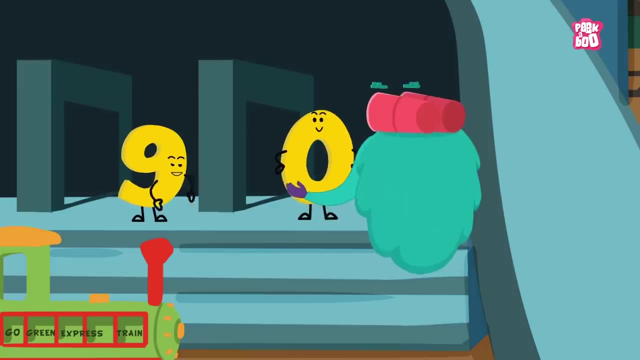 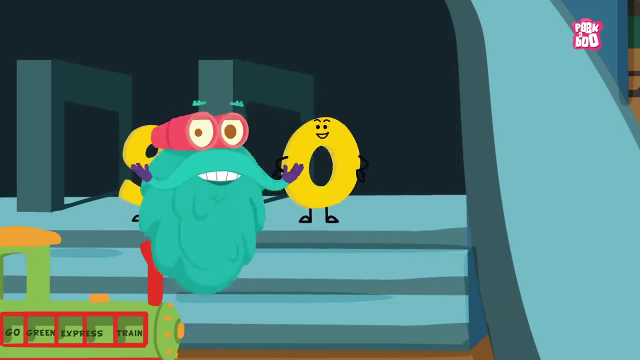 The number zero is neither negative nor positive. It's a natural number. Come, friends, let's take this zero back to our number collection. Oh, look at this, Isn't our zero looking beautiful? What? No way. Something is missing again.